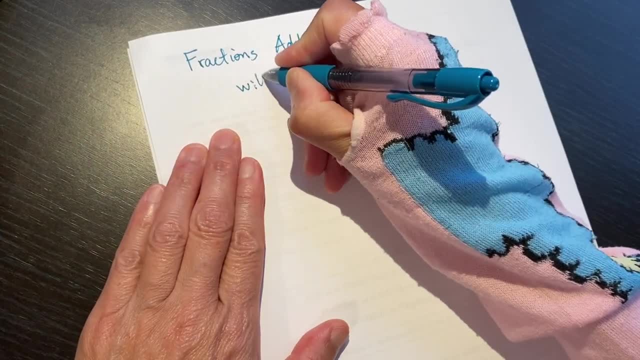 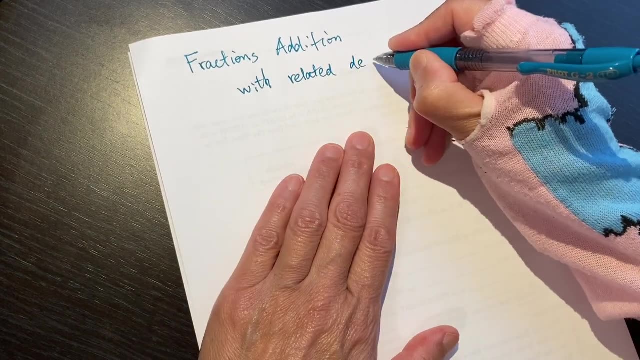 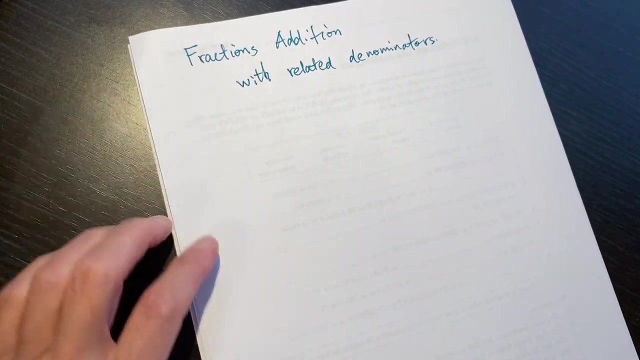 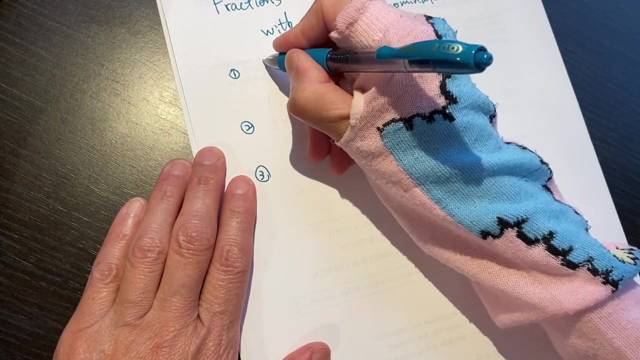 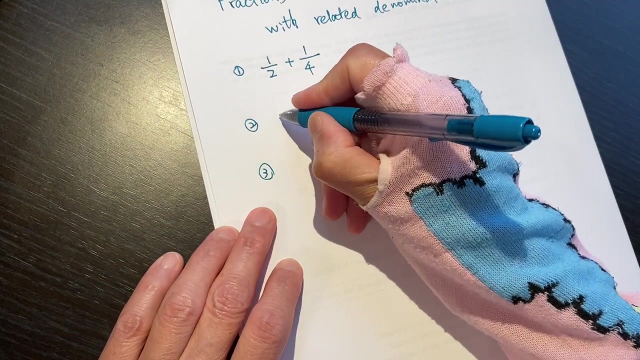 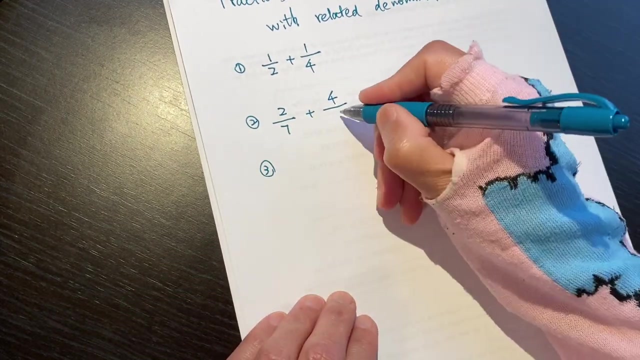 the same. So we learn fractions, addition with related denominators. So I will bring up three questions. The first one: 1 over 2 plus 1 over 4.. The second one: 2 over 7 plus 4 over 21.. 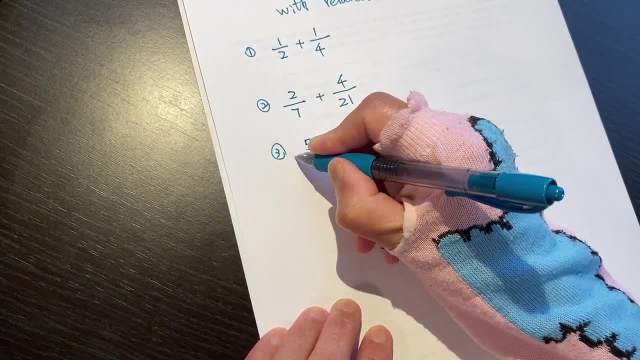 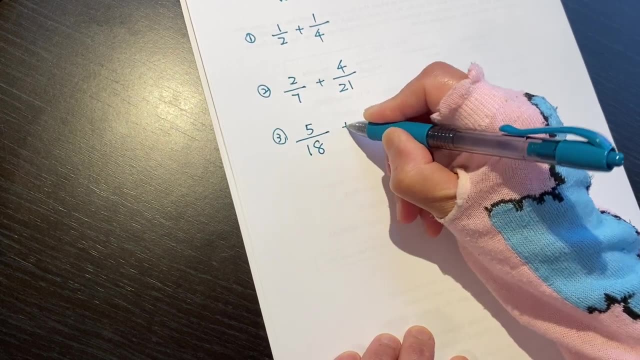 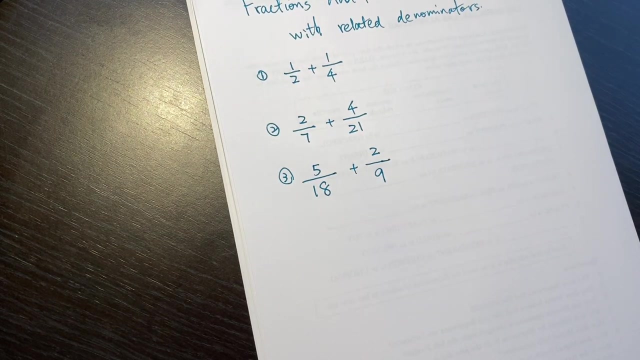 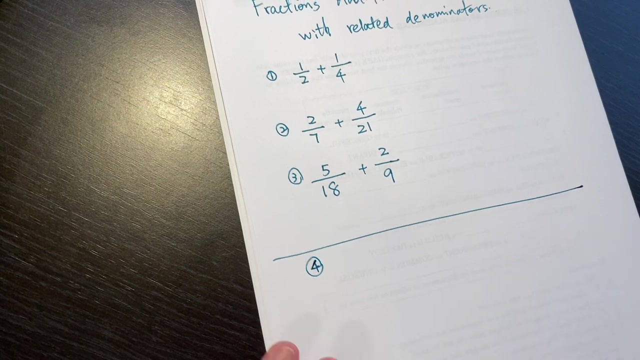 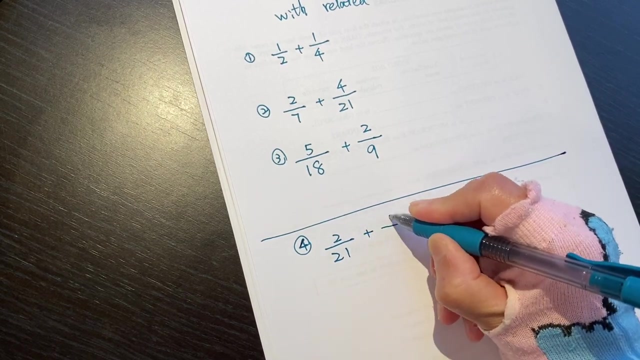 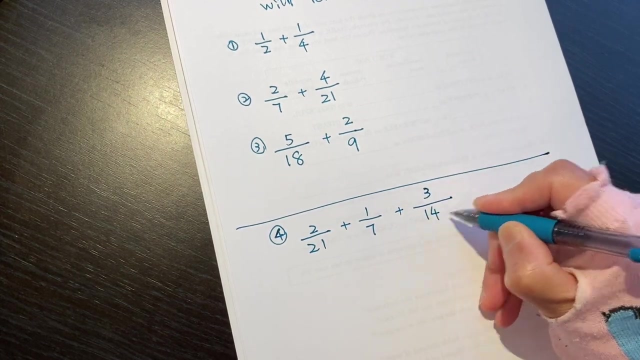 The third one: 5 over 18 plus 2 over 9.. Take a look, I will bring another challenge question. Question number 4 is a challenge. Okay, it's 2 over 21 plus 1 over 7, plus 3 over 14 plus 5 over 28.. 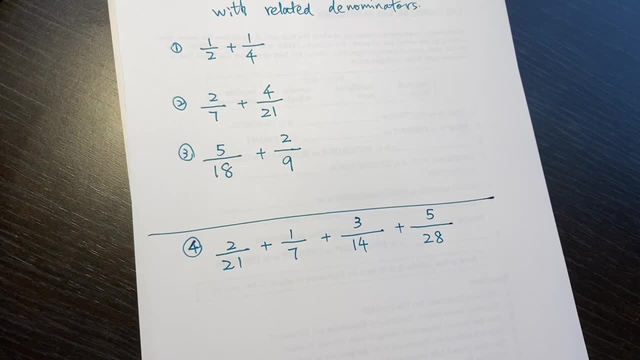 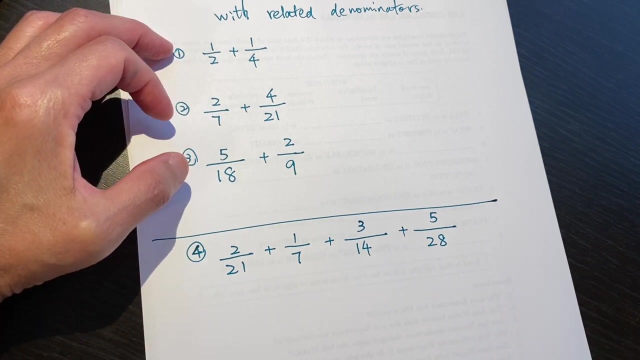 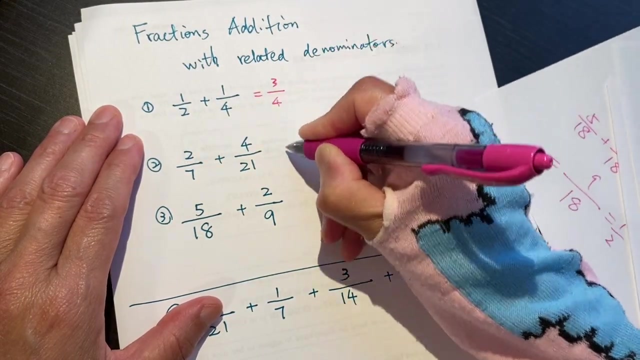 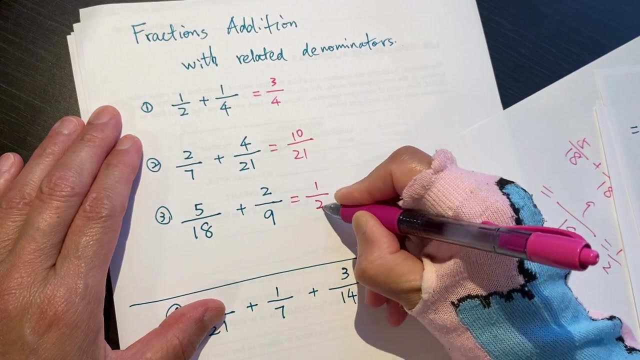 This is a challenge one. Okay, you can take a look. Turn it off, pause the video. I will let you see the result and then we will move on. Okay, so you can pause it. So here is the result: 3 over 4 and 10 over 21 and half, and. 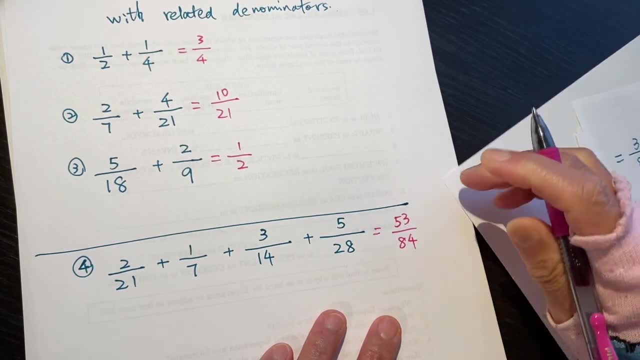 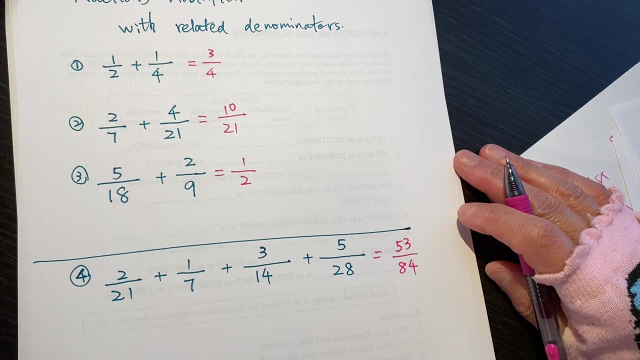 53 over 84.. If you get the same result, you are all good. No need to listen to me. Move on to the next lesson. If not yet, we keep on learning and I will explain step by step how I made it. 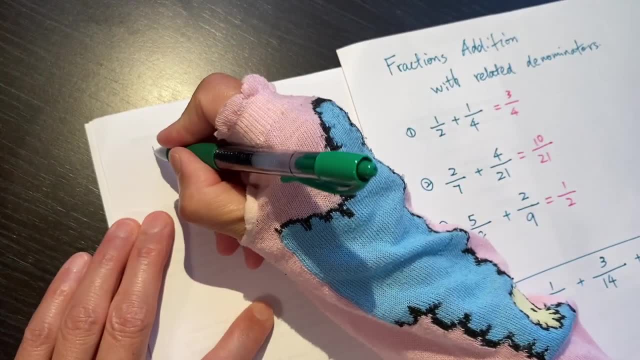 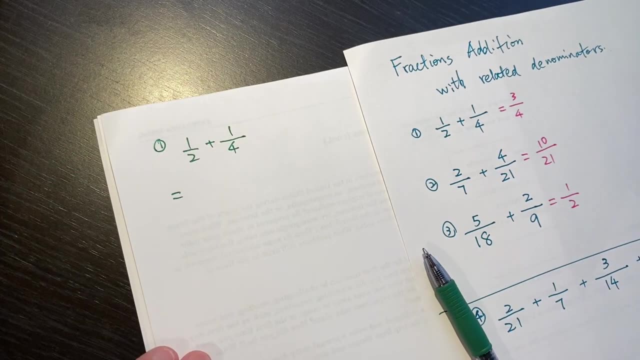 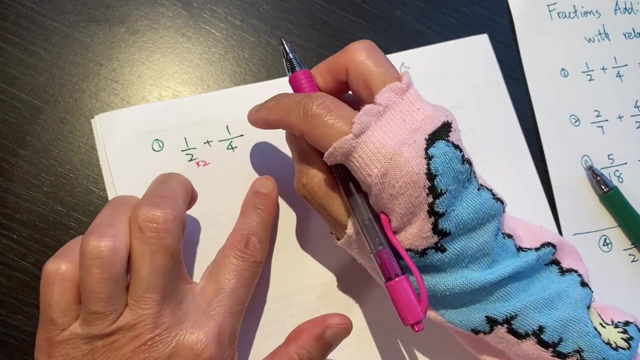 Okay. so the first question: how I did it? 1 over 2 plus 1 over 4.. The denominator is not the same. I need to make it the same: 2 times 2 makes 4, so the denominator means the same. 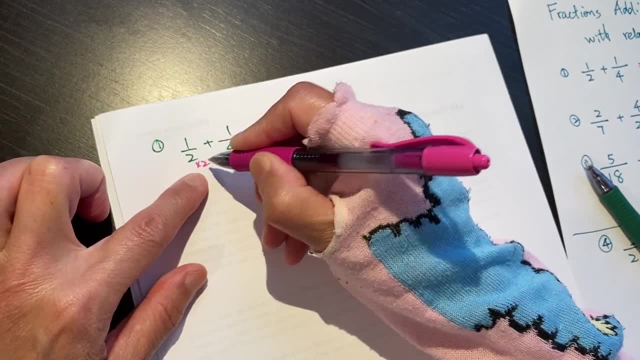 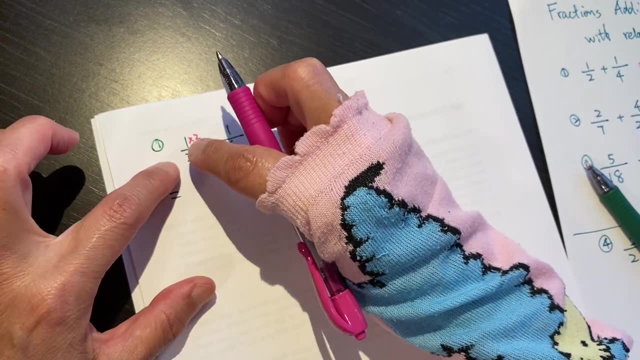 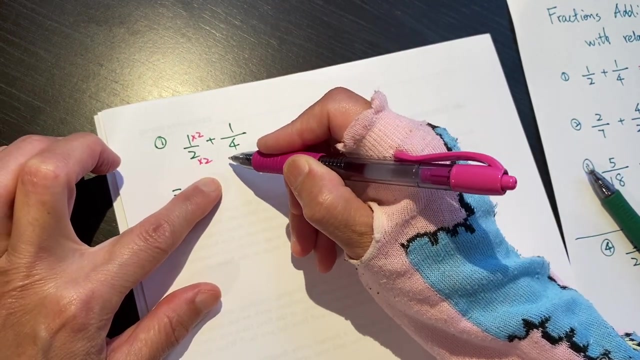 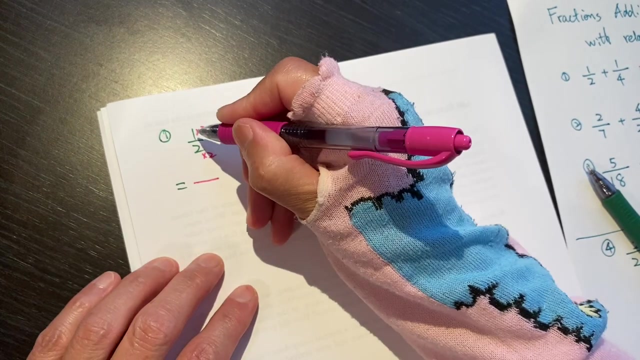 If for a number, I time a number on the bottom, I need to time exactly the same number at the top. In fraction, addition, subtraction, the denominator must must must not be the same number. Now. next is the obj must must be the same. Now I do the equivalent change: 1 times 2 is 2.. 2 times 2 is 4.. I did not. 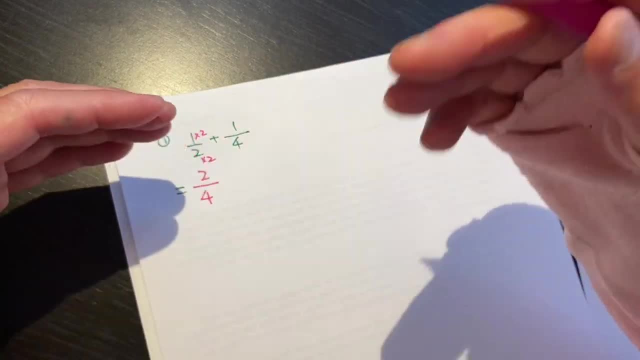 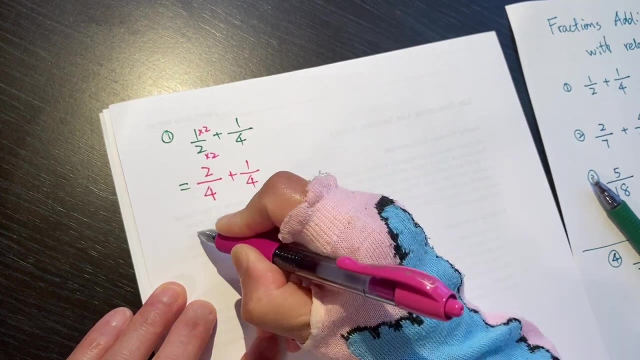 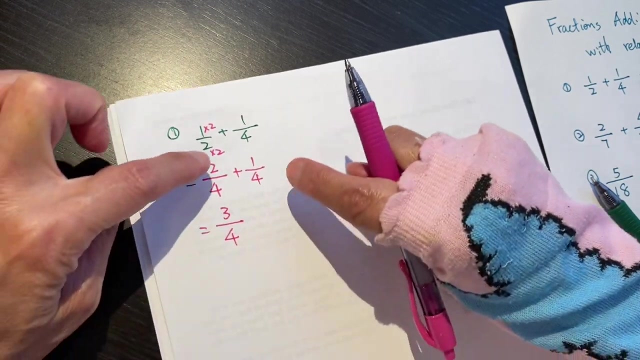 change the number. I only write it a different way, but the true value is the same, Plus 1 over 4,, which is 3 over 4.. The bottom, the denominator, do not change, And the operation is to add the. 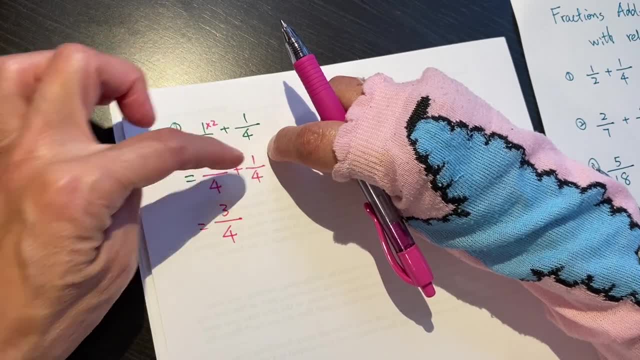 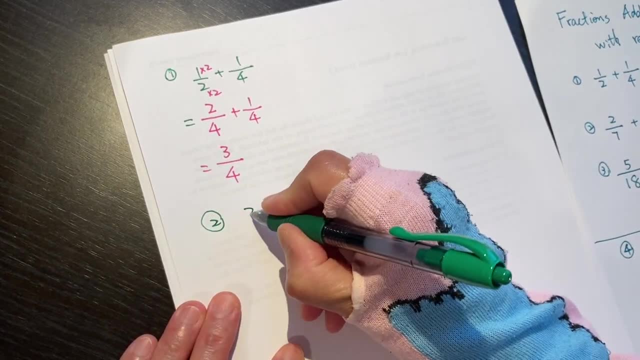 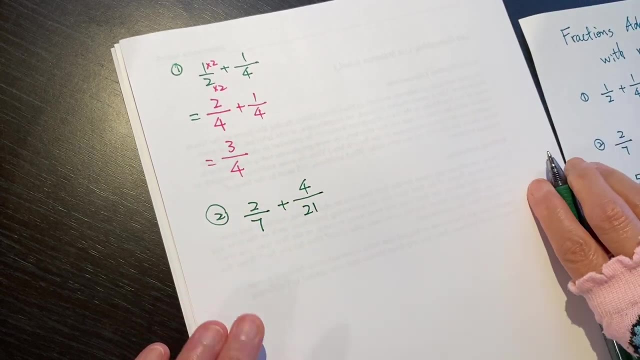 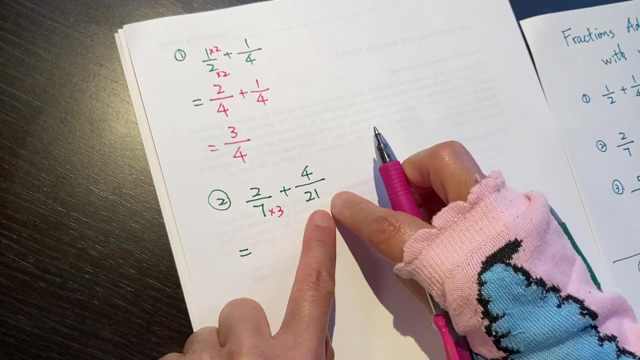 top number, the numerator 2 plus 1 is 3.. Okay, so this is how we get the answer. The second one: 2 over 7 plus 4 over 21.. They are not the same number. So 7 times 3 makes 21.. If on bottom we times 3, on top we need to times 3.. So 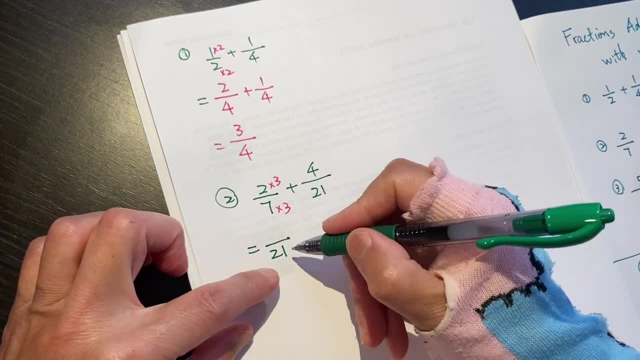 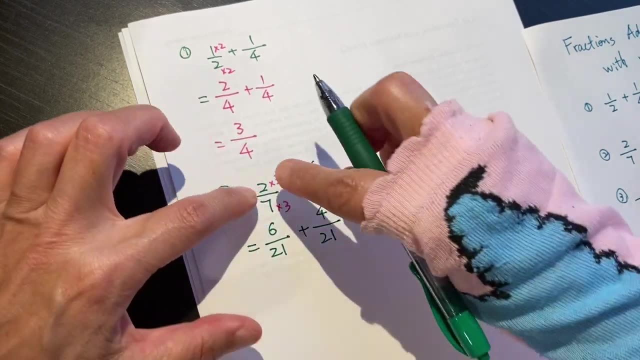 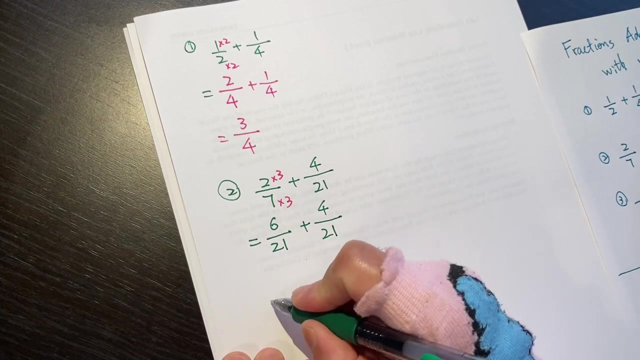 that one we get 21 on the bottom and on top is 6 plus 4 over 21.. Exactly the same number. Change a way of writing, but it's equivalent. change The second one: 2 over 7 plus 4 over 21.. They are not. 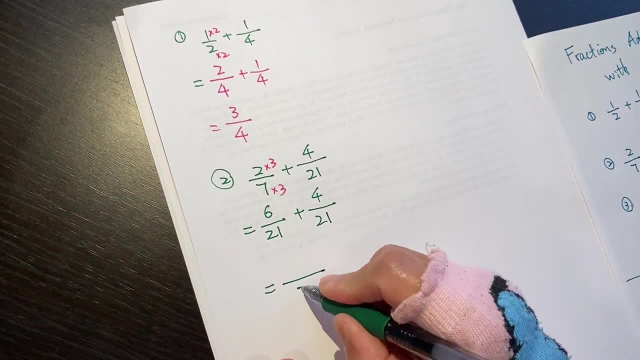 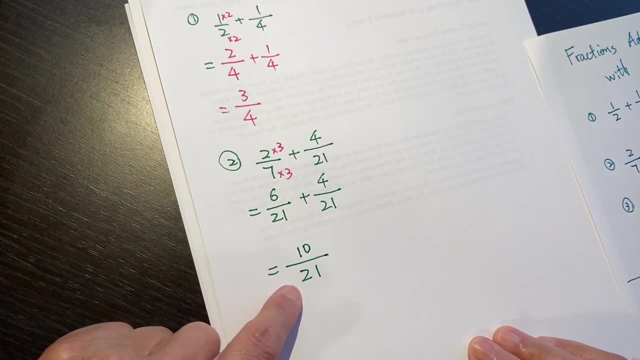 the same number, So 7 times 3 makes 21.. They are not the same number, So 7 times 3 makes 21.. They change, So the bottom is the same, Never change 21.. And the top 6 plus 4 is 10.. This is how we. 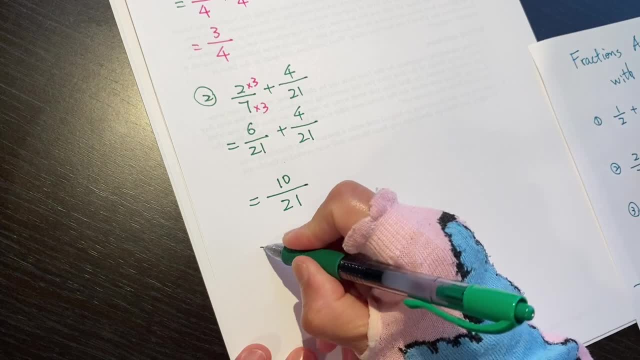 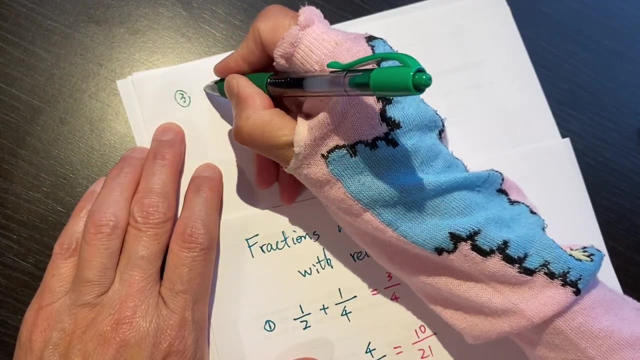 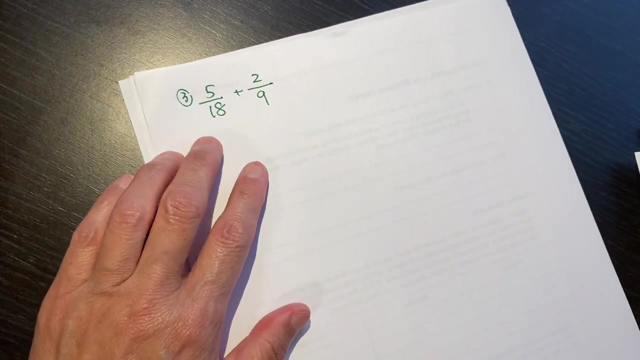 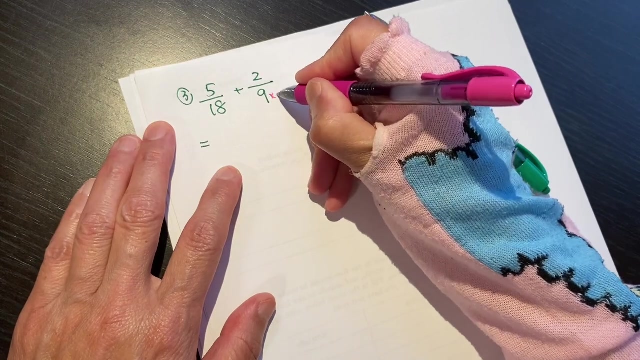 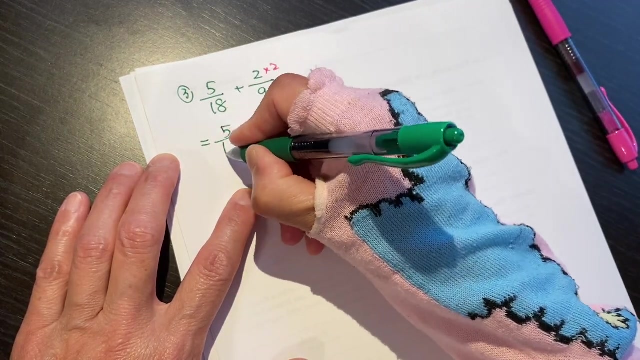 get this answer. Now the third one. Okay, the third one: 5 over 18 plus 2 over 9.. We can see the bottom is not the same, so we need to make it the same: 9 times 2, 18 times 2 times 2, so it becomes 5 over 18. 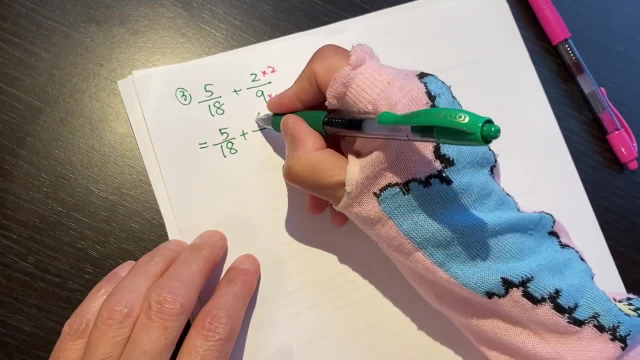 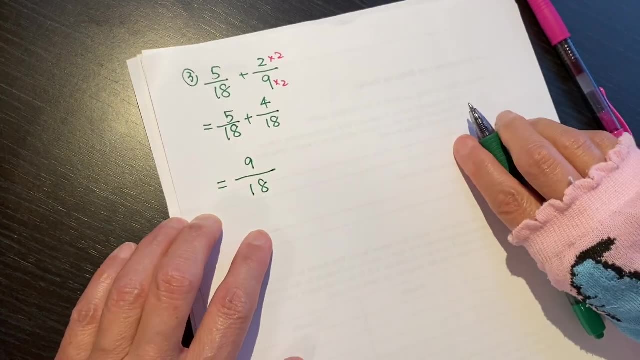 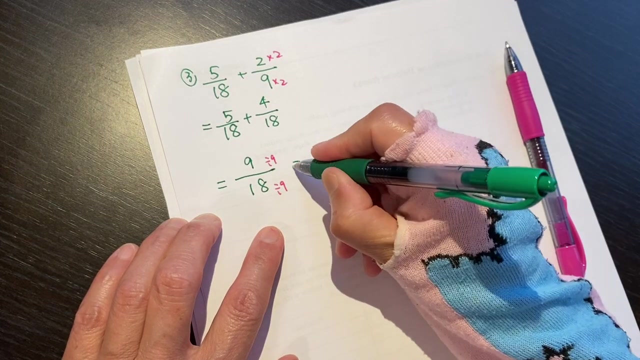 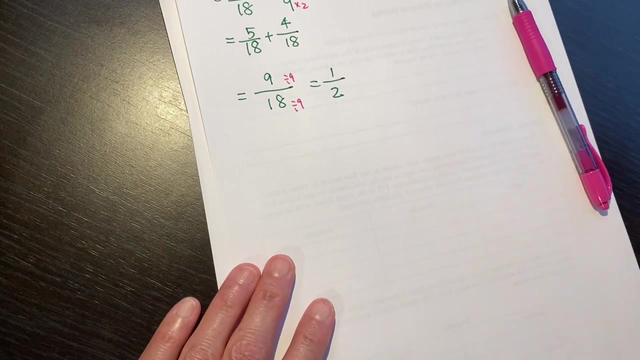 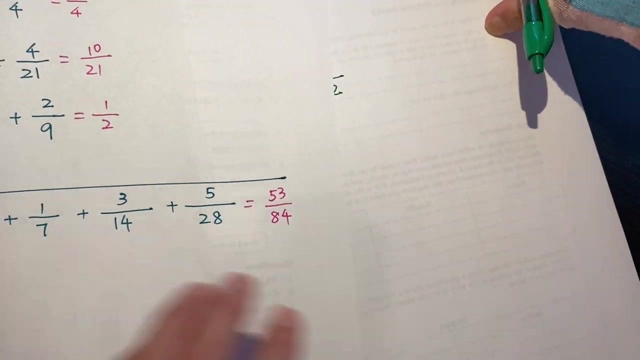 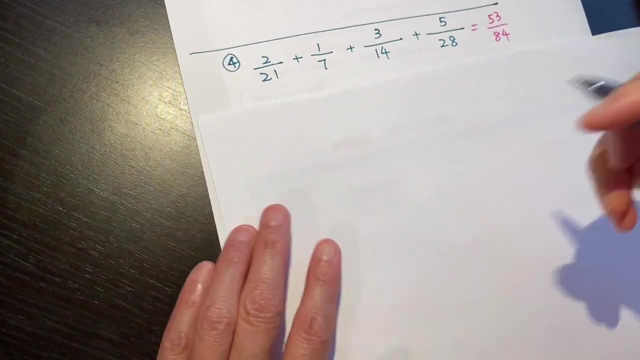 we do not change plus 4 over 18, which makes 9 over 18. we can simplify both divided by 9, which makes 1 over 2, which is half, as we have got okay. the last one is a little bit complicated right now. I will do it. I use a paper with this way: write it large enough, okay, question. 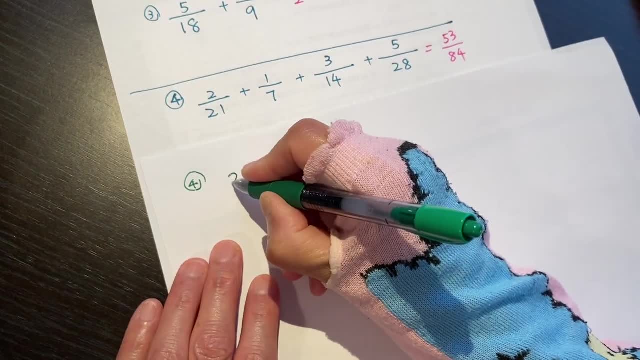 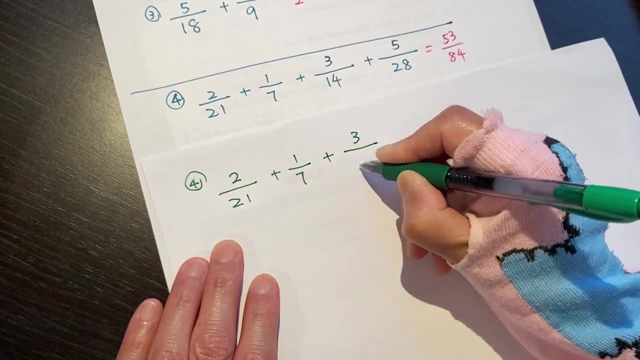 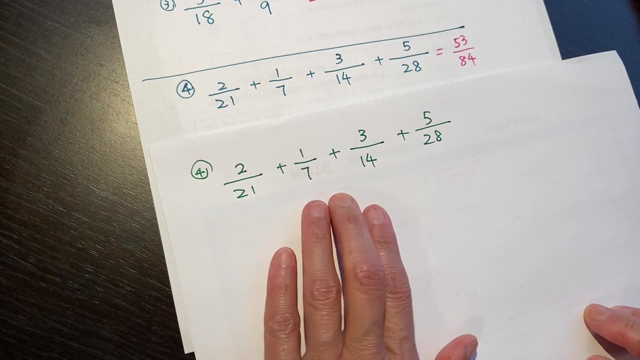 number four. you can see it right: two over 21, plus 1 over 7, plus 3 over 14, plus 5 over 28. it is hard to find the relationship of all these, but we can see what we can see. they are all three multiples of 7, so we can. 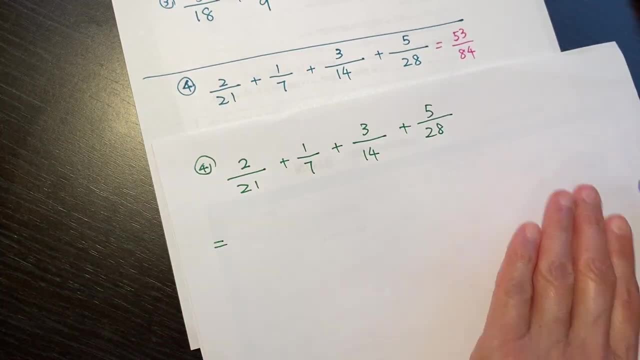 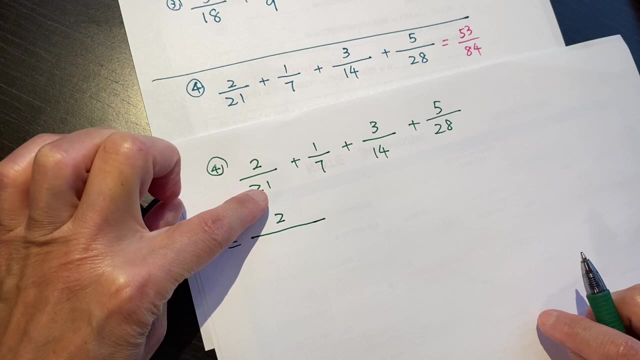 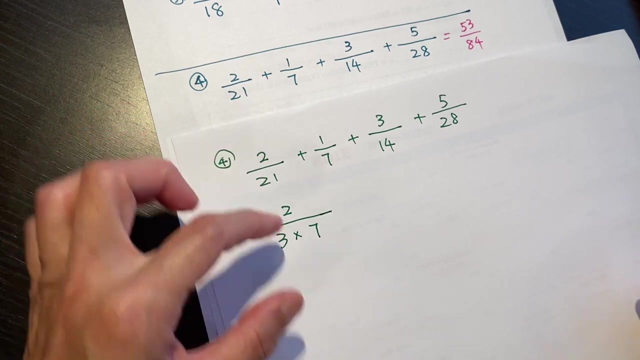 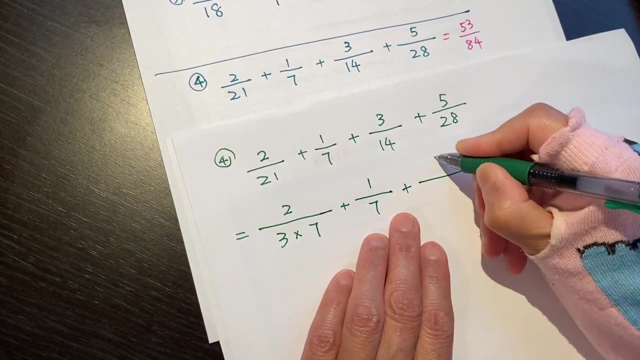 write it in another way: on top is 2 and on the bottom we can write 21 as 3 times 7. I did not change, still the same number. and the second one, 1 over 7. the third one, 3 over 2 times 7. it is: 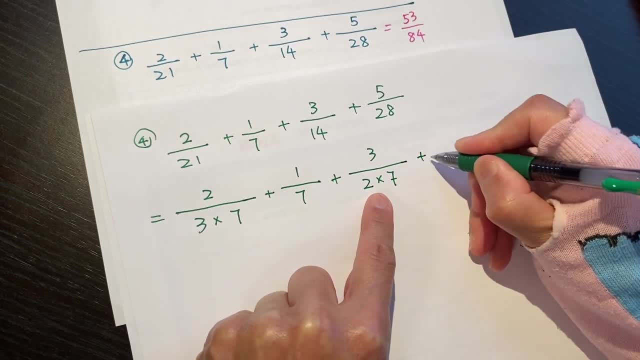 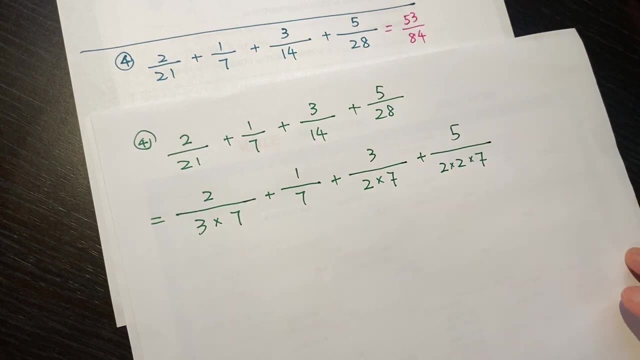 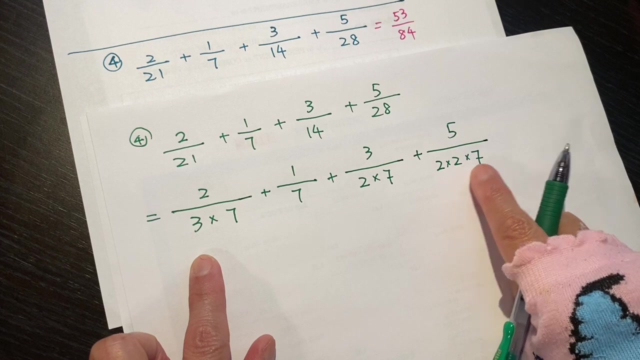 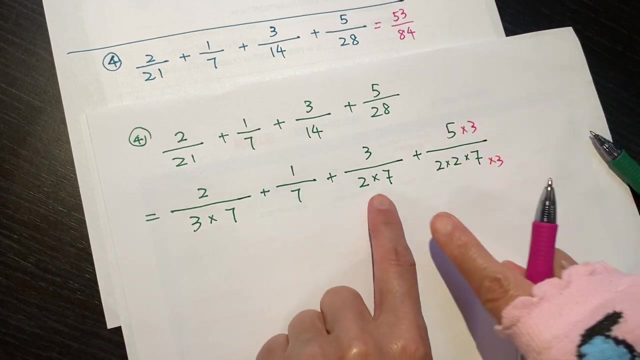 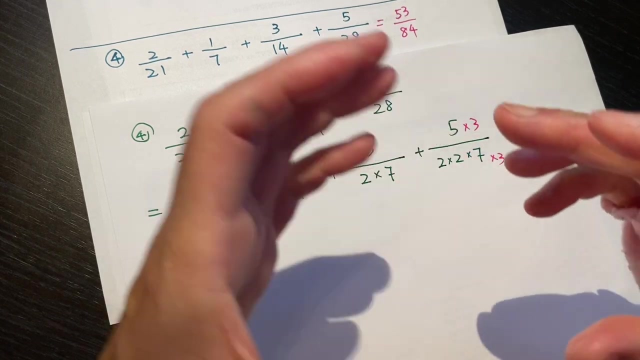 the same number I write differently. Why do I do this? 5 over 2 times 2 times 7? I write it so that we can see this: 2, 2, 7. if I times 3 times 3 and this one, so I have 2, 2, 7, 3, this one, two, three, four, four factors. 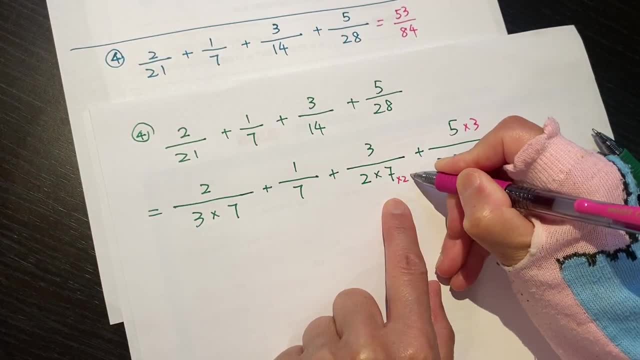 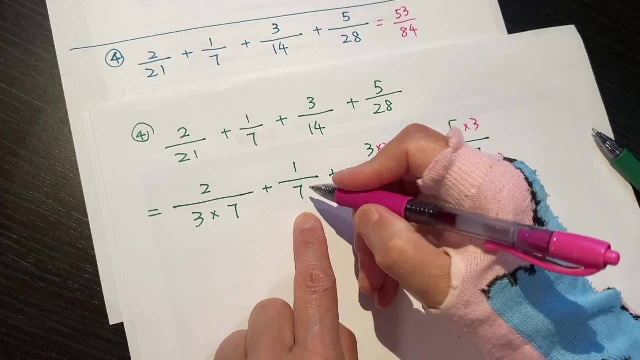 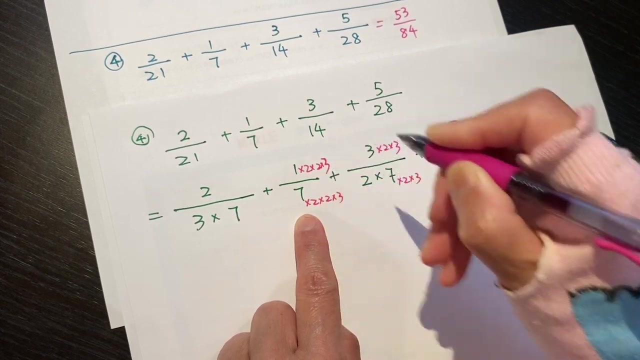 Now we have only two factors need to time 2 times 3 times 2 times 3. this one, only one factor. so we need to time 2 times 2 times 3 times 2 times 2 times 3, which is 12. this